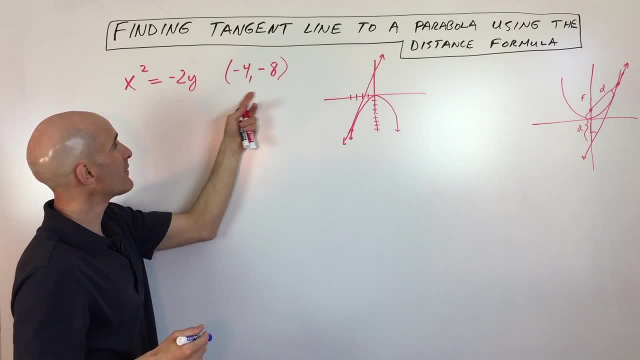 show you what I mean in this example. So here what we want to do is we want to find the equation of the tangent line okay to this parabola: x squared equals negative 2y, through the point negative 4,, negative 8.. So I've drawn a little sketch here for us, just so we can see it a little. 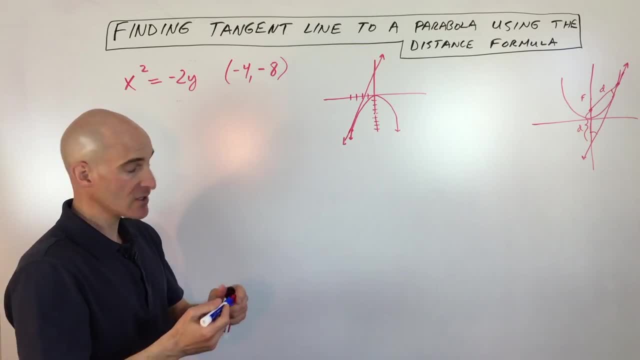 bit better, And so what we're going to do first thing is we're going to find the focus. So, if you notice, this is in the form: x squared equals 4py, And if you need to reference how to graph parabola, you can do that here. So I'm going to do that here. So I'm going to do that here, And 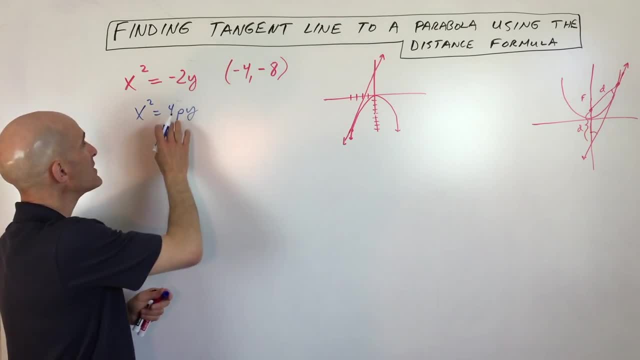 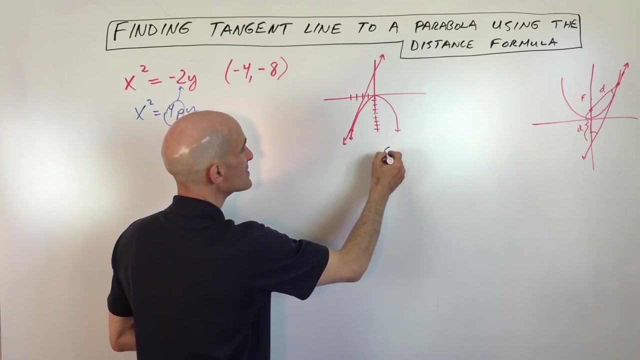 you can. I'll have a link for the video for that. But basically you can see that 4p equals negative 2. So that means that p equals negative one half right. So if we go down here, this is going to be negative one half, right there. Okay, that's our focus. So the focus is at 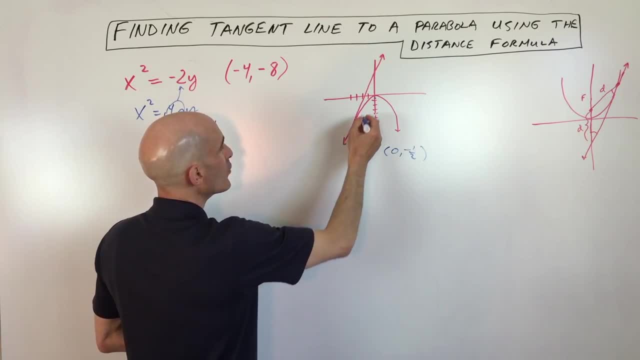 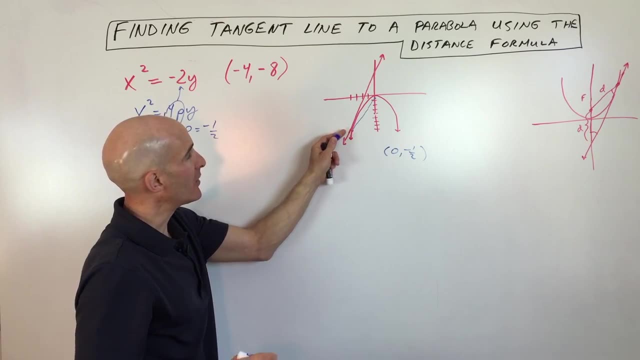 zero comma negative one half. And we want to find the distance from that point to the point where the tangent line just barely touches the parabola. Okay, and this point over here is negative 4, negative 8.. So what we're going to be doing is we're going to be doing the 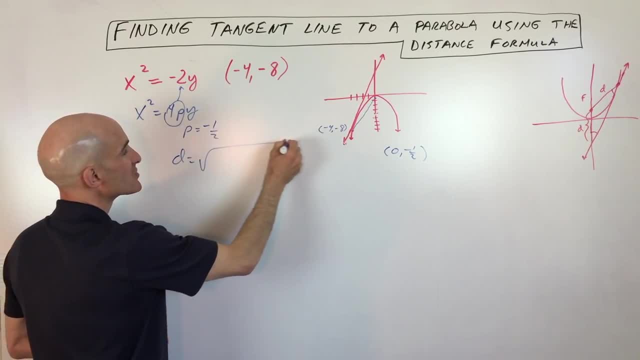 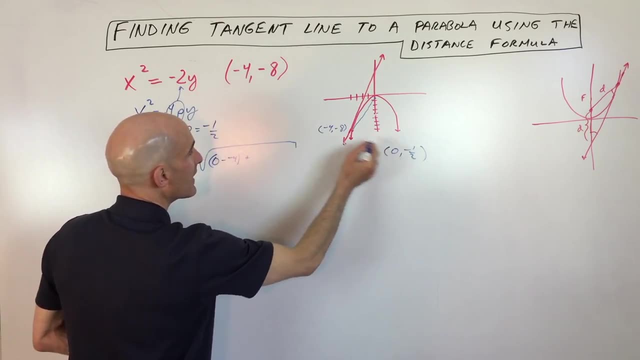 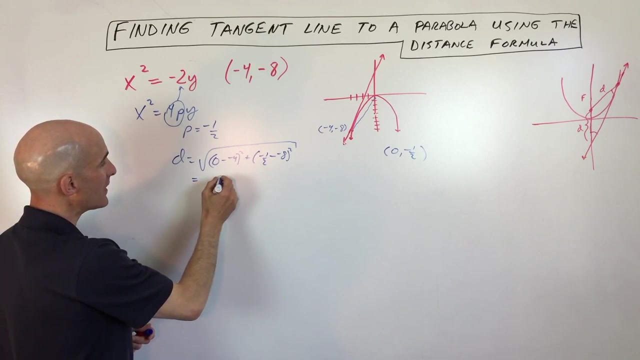 distance formula. So let's go ahead and do that. So we have: the distance equals the square root of zero minus negative, 4 squared, plus negative one half minus negative 8 squared. Add those together and take the square root. So if we simplify this, we get 16 plus. this comes out to: 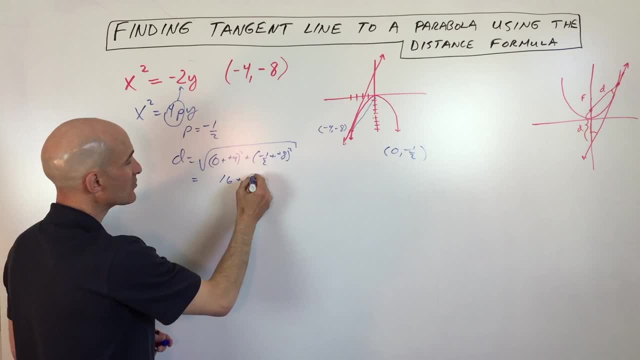 seven and a half, which is 4py, And we're going to do that here. So if we simplify this, we get 15 halves, which if we square that, we get 225 fourths. And if we get common denominators here, 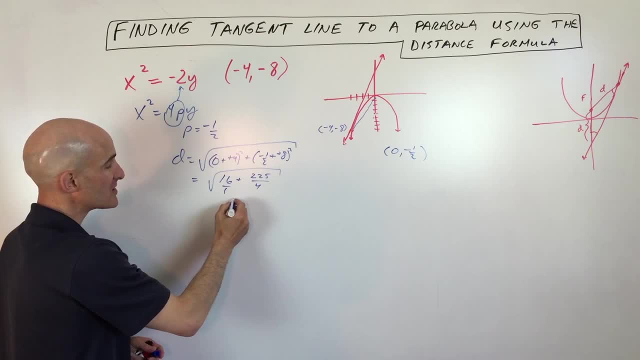 this is 64 fourths plus 225 fourths is 289 fourths, And if we take the square root of that, we're going to get 17 over 2, which is 8 and a half Okay. so what that means is that this: 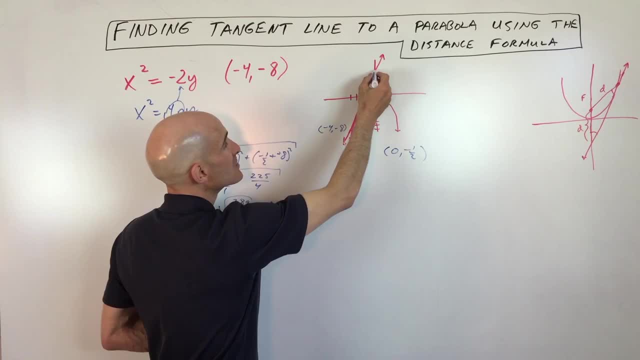 distance here is 8 and a half. The distance from the focus to the y-intercept: okay, that the tangent line crosses the y-axis over here. this distance is also going to be 8 and a half And because the focus is over here, a half unit.